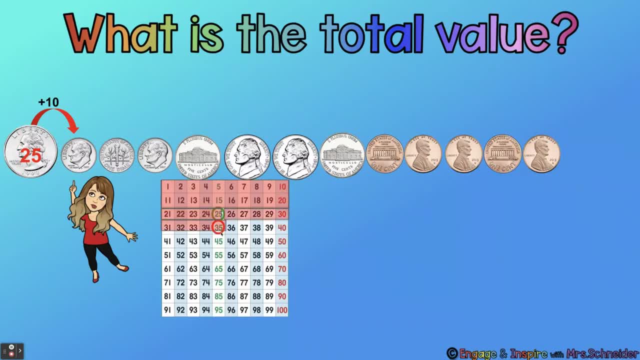 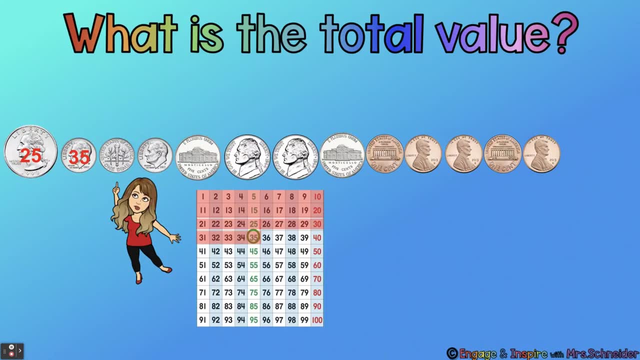 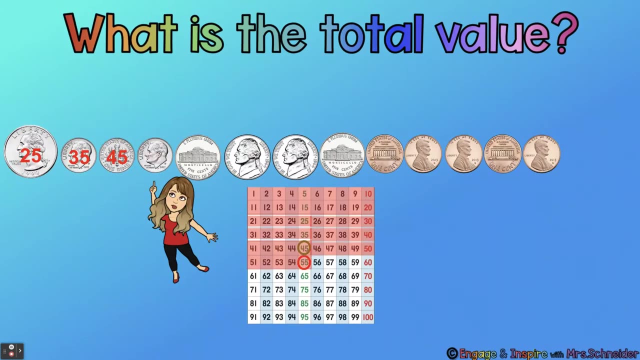 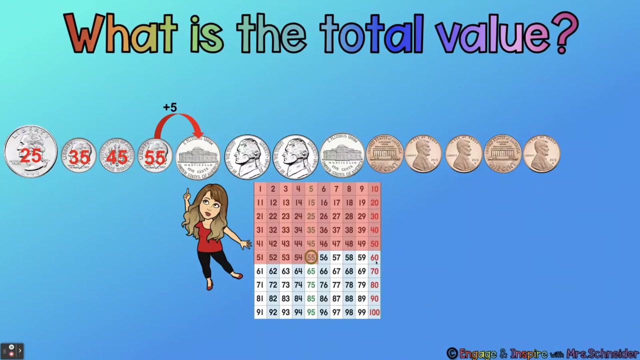 what's it gonna be? 35,, good, Okay, and 35 plus 10 is 45.. 45 plus 10 is 55.. Now we're going to count by fives. So 55 plus five more is 60.. 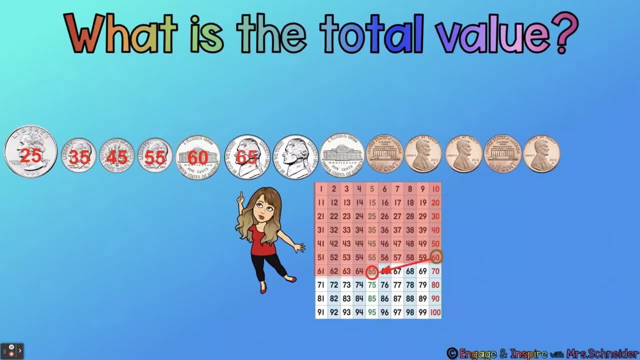 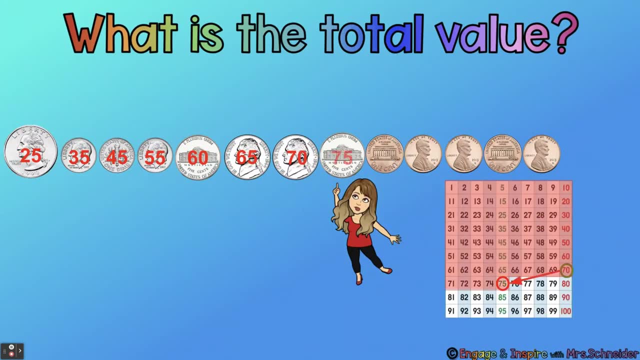 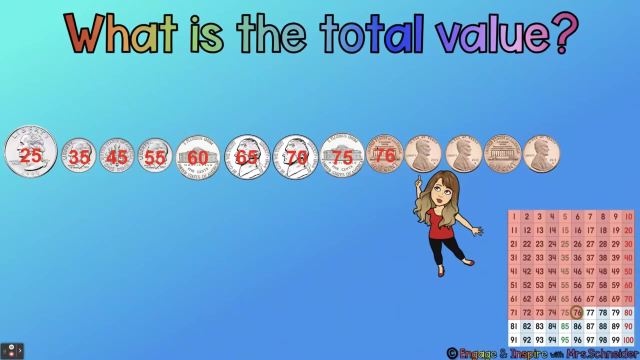 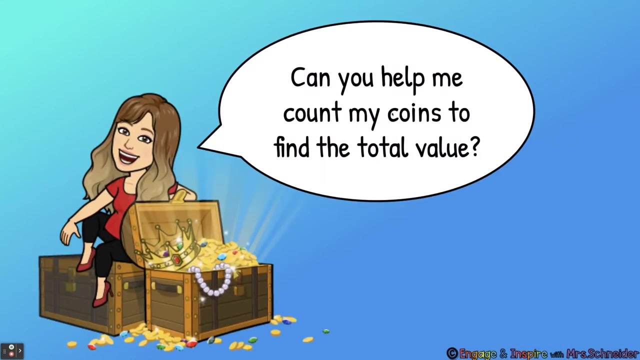 65, 70,, 75.. And now we're gonna count by ones. So 75 plus one is 76,, 77,, 78.. 78, 79, 80.. Can you help me count my coins to find the total value? 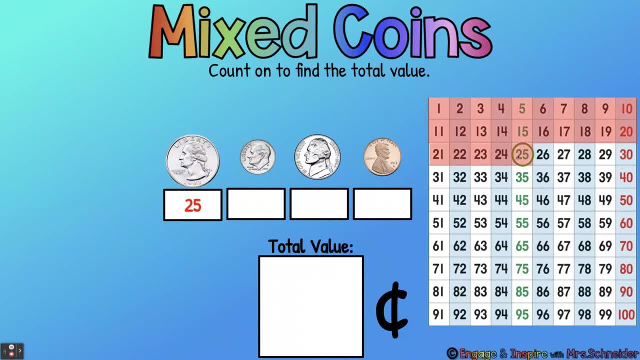 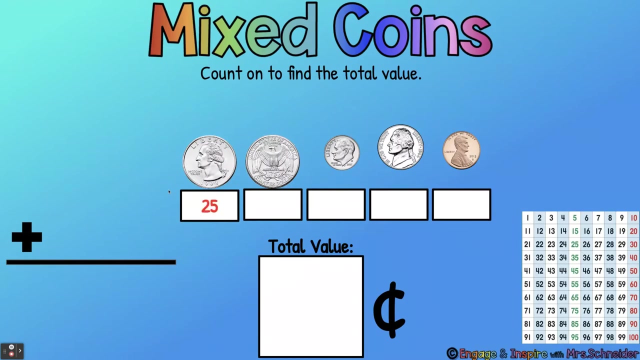 One quarter is 25 plus 10,, 35 plus five, 40. And one more 41,, so we have 41 cents here. good job, Let's count these coins. One quarter is 25,. two quarters is 50. 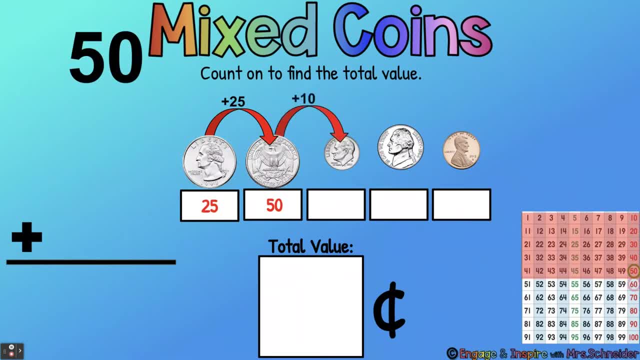 So 50 cents plus 10,, 60, plus five more 65, plus one more 66.. Let's look at that over here: Zero plus zero, So five plus one is six, and five plus one is six, 66.. 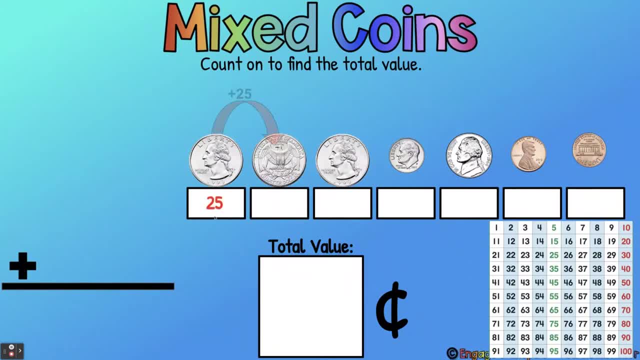 Good job, let's do another one. One quarter is 25,, two quarters is 50,, three quarters is 75,, 75 plus 10,, 85,, 85 plus five is 90. And 90 plus one is 91,. 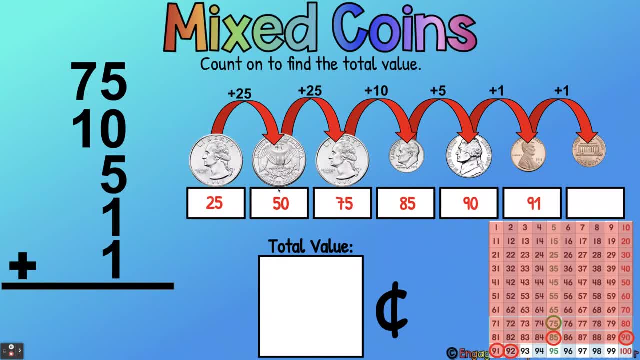 plus one more is going to be 92. And we look over here we have five plus five is 10,, plus one more is 11, and one more is 12.. But we can't write a 12 in the ones place. 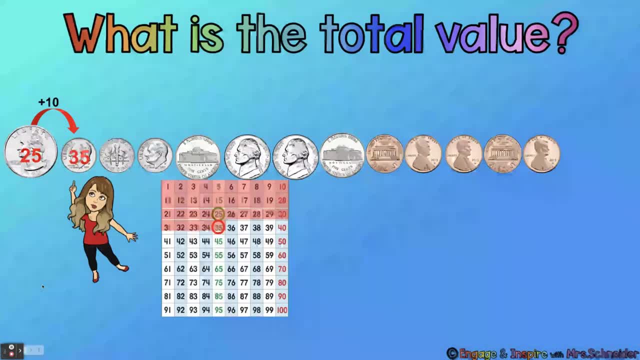 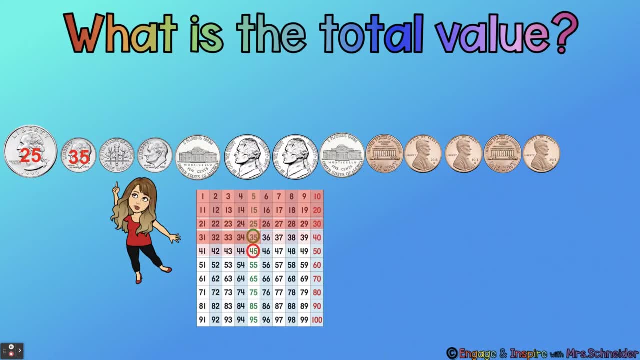 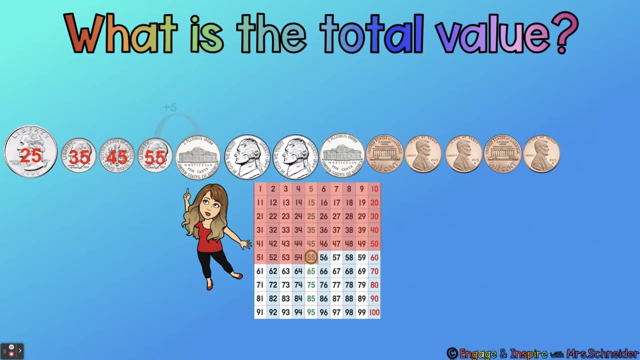 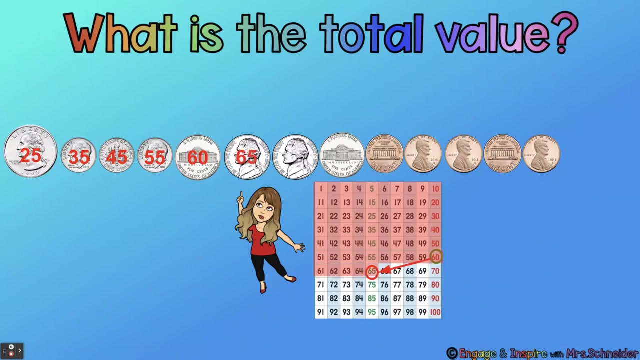 35.. Good, Okay, and 35 plus 10 is 45.. 45 plus 10 is 55.. Now we're going to count by fives. So 55 plus 5 more is 60.. 65., 70.. 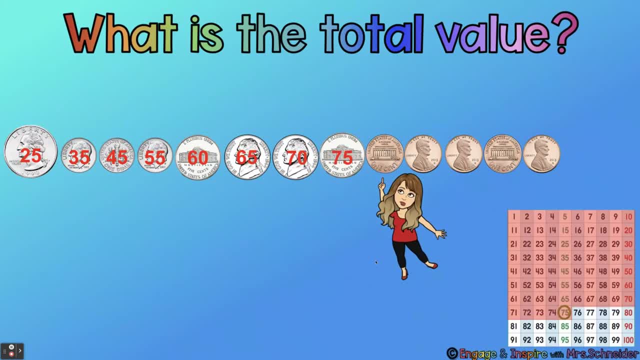 75.. And now we're going to count by ones. So 75 plus 1 is 76., 77., 78., 79., 80.. Can you help me count my coins to find the total value? One quarter is 25.. 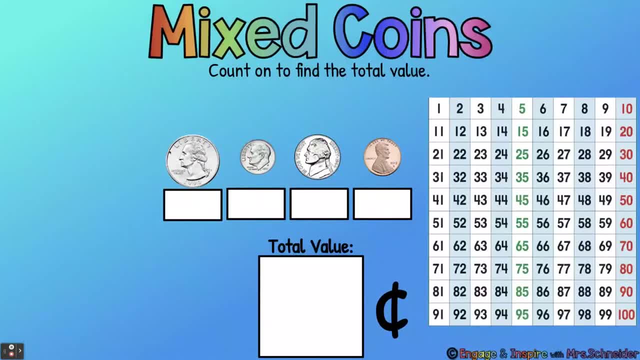 Plus 10.. 35. Plus 5., 40., 40., 75., 75., 80., 40. And one more, 41. So we have 41 cents here. Good job, Let's count these coins. 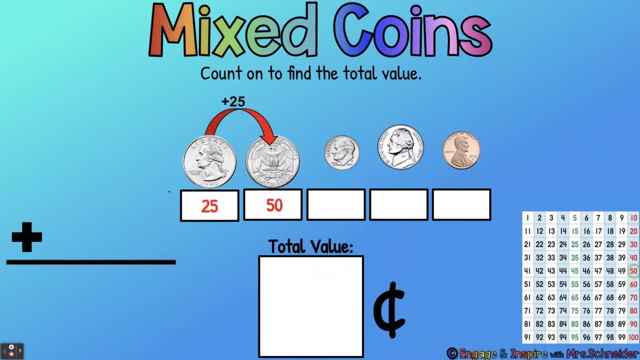 One quarter is 25.. Two quarters is 50. So 50 cents Plus 10. 50.. 60. Plus 5 more 65. Plus 1 more 66. Let's look at that over here. 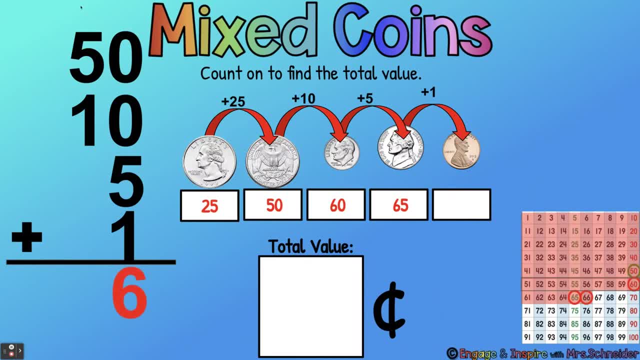 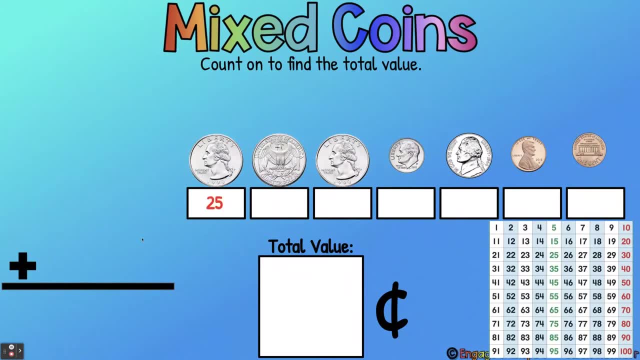 Zero plus zero. So 5 plus 1 is 6. And 5 plus 1 is 6.. 66.. Good job, Let's do another one. One quarter is 25.. Two quarters is 50.. Three quarters is 75.. 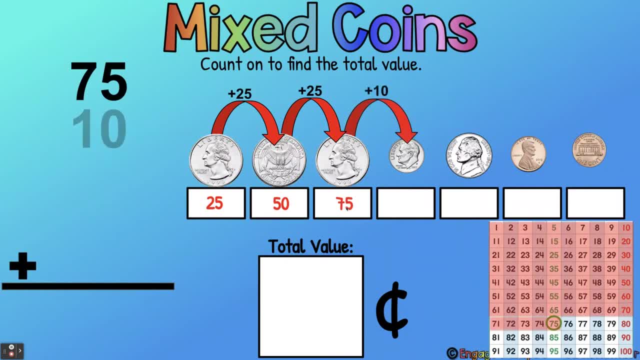 75. Plus 10.. 85., 85. And 85. Plus 5. Is 90. And 90. Plus 1. Is 91. Plus 1 more Is going to be 92. And we look over here. 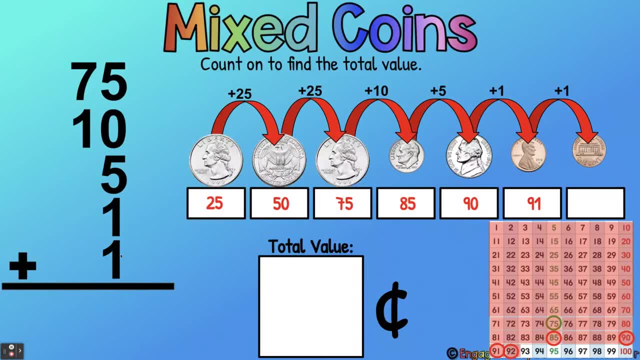 We have: 5 plus 5 is 10.. Plus 1 more is 11. And 1 more is 12.. But we can't write a 12 in the ones place, So we're going to put the 2 down here. 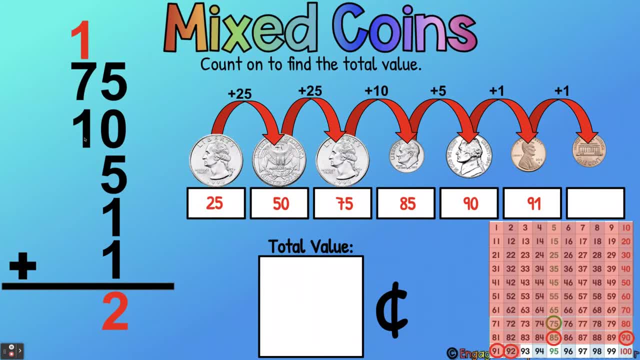 And carry the one 10 up top, And then 1 plus 7 plus 1 is 9.. So our answer is 92 cents. Good job. What do you like most? Do you like adding? Do you like counting on? 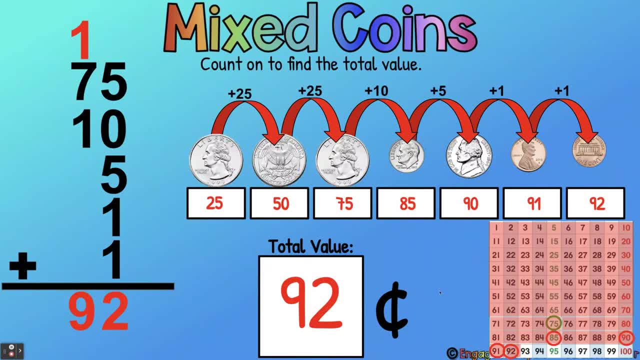 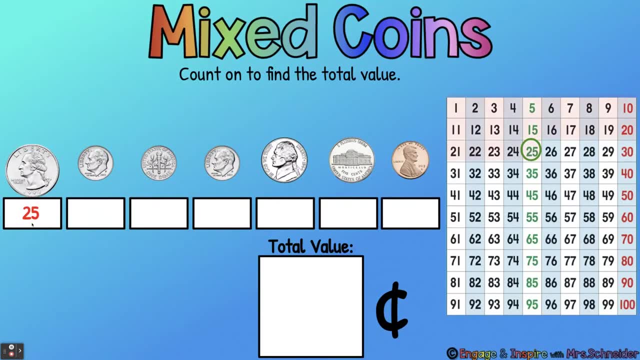 Or do you like using the numbers chart, Let's count another one. One quarter is 25. Plus 10. Is 35.. 35. Is 35. Is 35. Plus another 10.. 45. Plus another 10.. 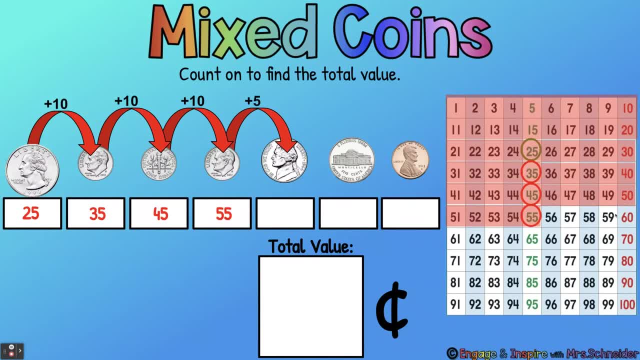 55. And 55 plus 5.. Now we can count by 5's Right: 55 plus 5 is 60. And 60 plus 5 is 65. And 60 plus 5 is 65. And 60 plus 5 is 65.. 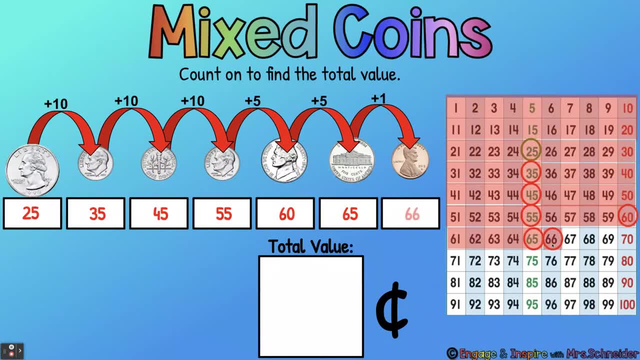 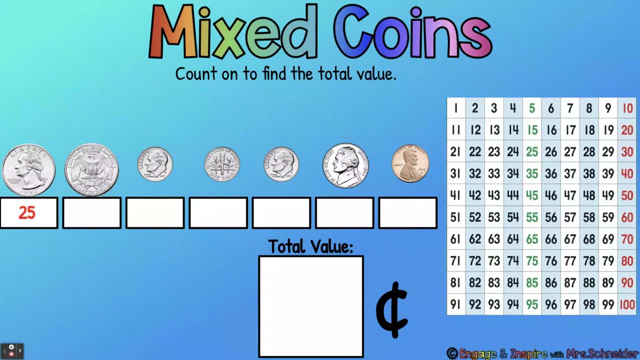 65 plus 1 more is 66.. 65 plus 1 more is 66.. Good job, Here we go. One quarter is 25.. Two quarters is 50.. Two quarters is 50.. Here's 50 on our hundreds chart. 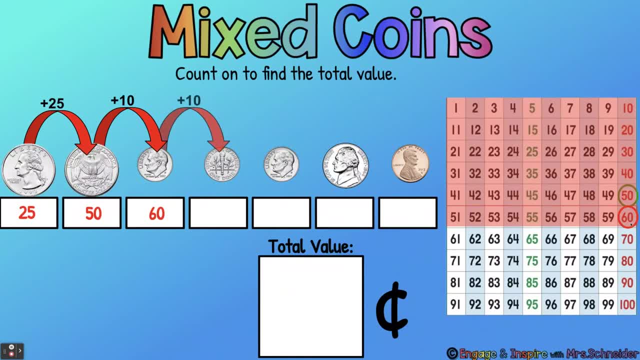 We're going to add 10. 60. Plus another 10. 70. Plus another 10. 80. And 80 plus 5.. 1,, 2,, 3,, 4,, 5. Is 85.. 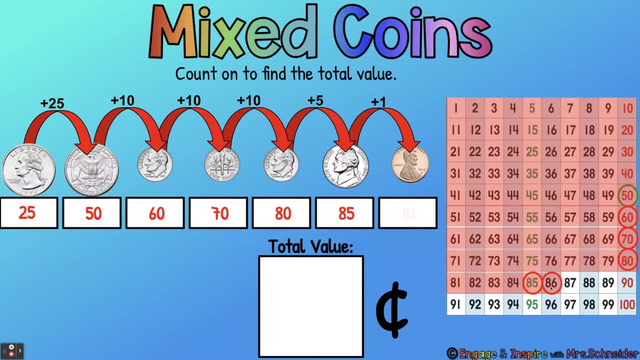 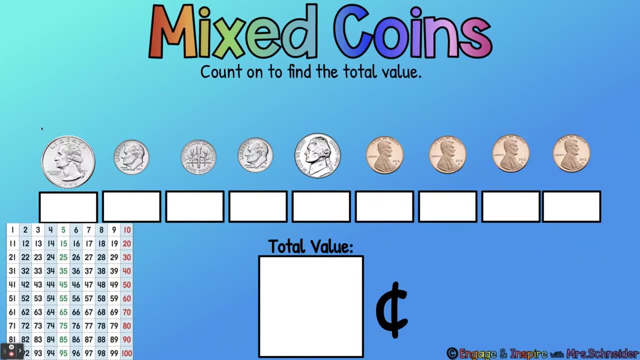 Plus one more, 86.. The total value of these coins is 86 cents. The total value of these coins is 86 cents. Are you ready for another one? Count out loud with me. One quarter is 25.. Here's 25 on our chart. 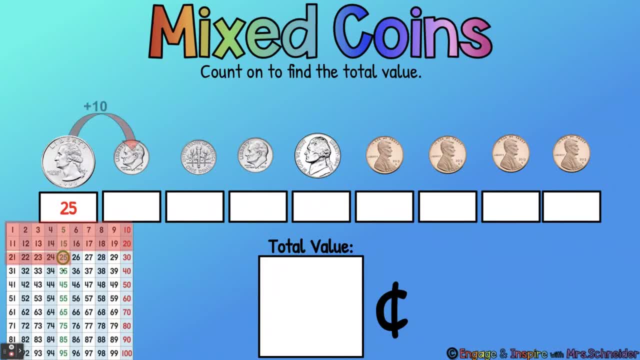 We're going to add 10.. You know what that means. Plus 10 is 35.. Plus another 10 is 45.. Plus another 10 is 55. Plus another 10 is 55. And then we're going to add 5.. 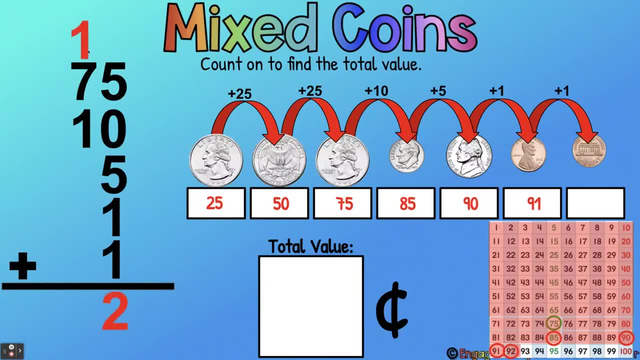 So we're gonna put the two down here and carry the one 10 up top, And then one plus seven plus one is nine. So our answer is 92 cents. Good job, What do you like most? Do you like adding? Do you like counting on? 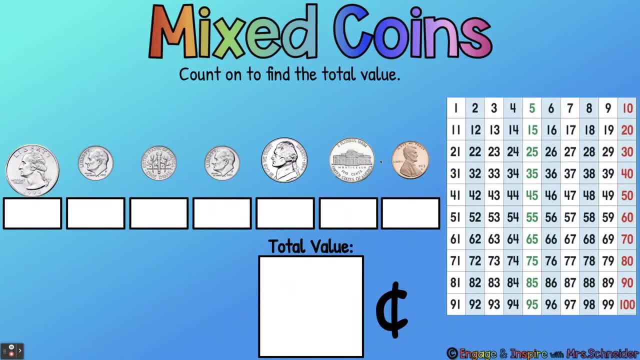 Or do you like using the numbers chart, Let's count another one. One quarter is 25 plus 10 is 35. Plus another 10, 45, plus another 10, 55. And 55 plus five. now we can count by fives, right. 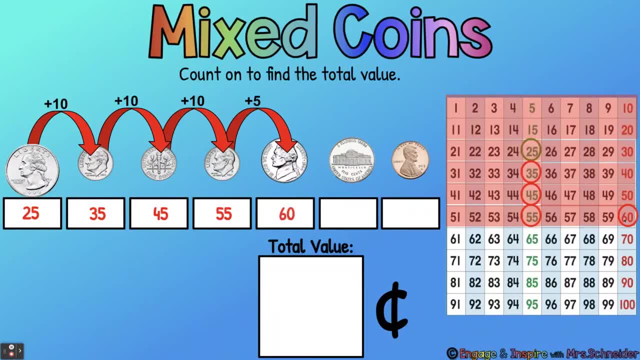 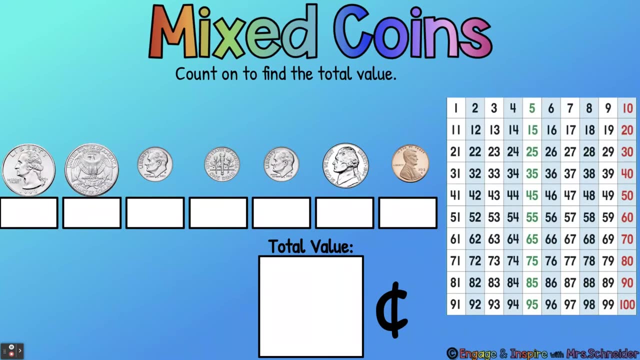 55 plus five is 60. And 60 plus five is 65.. 65 plus one more is 66.. Good job, Here we go. One quarter is 25.. Two quarters is 50.. Okay, here's 50 on our hundreds chart. 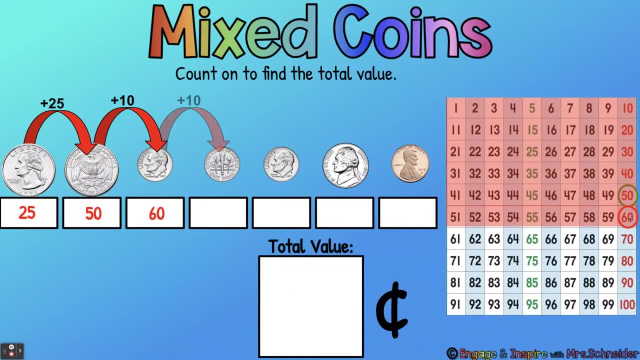 We're gonna add 10, 60, plus another 10, 70,, plus another 10, 80. And 80 plus five, one, two, three, four, five is 85. Plus one more 86.. 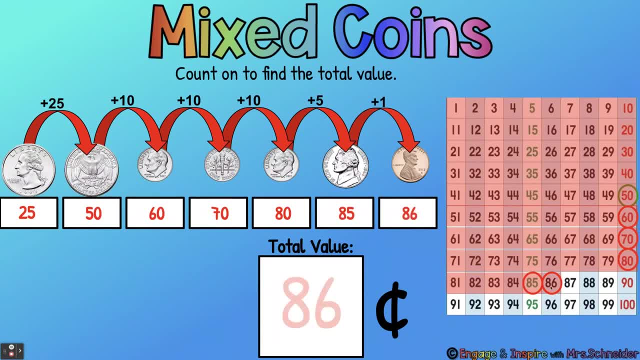 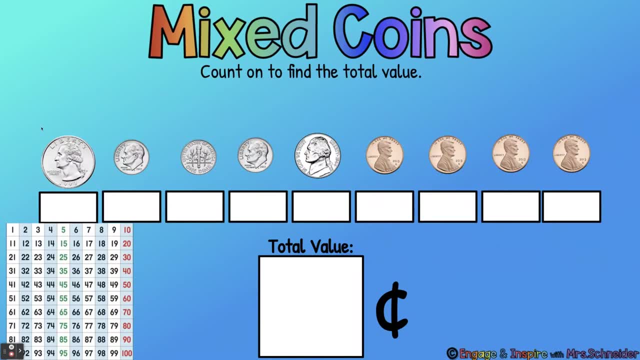 The total value of these coins is 86 cents. Are you ready for another one? Count out loud with me. One quarter is 25.. Here's 25 on our chart. We're gonna add 10.. You know what that means. 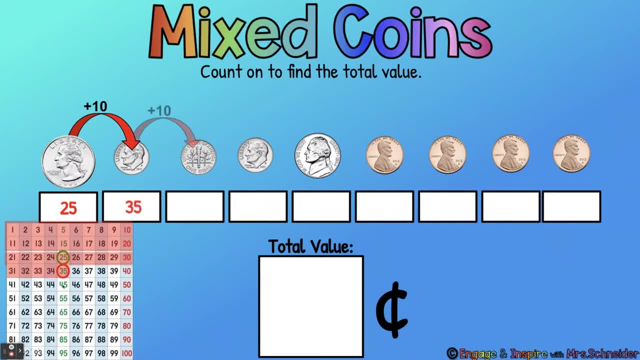 Plus 10 is 35. Plus another 10 is 45. Plus another 10 is 40. Look at that. plus another 10 is 55. Now we're going to add 5.. So 55 plus 5 is 60. And 60 plus 1 is 61,. 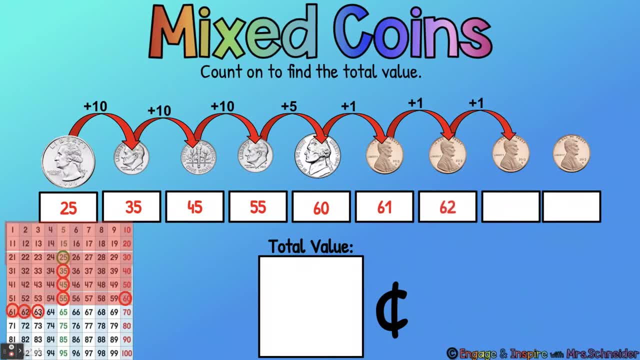 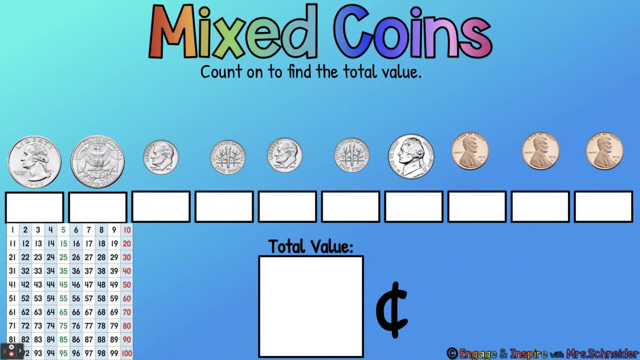 62,, 63,, 64. So our total value of these coins is 64 cents. Okay, here's another one. Are you guys having fun yet? One quarter is 25.. Two quarters is 50. Okay, here's 50 on our chart. We're going to add 10.. 50 plus 10 is 60, plus 10 more is 70,. 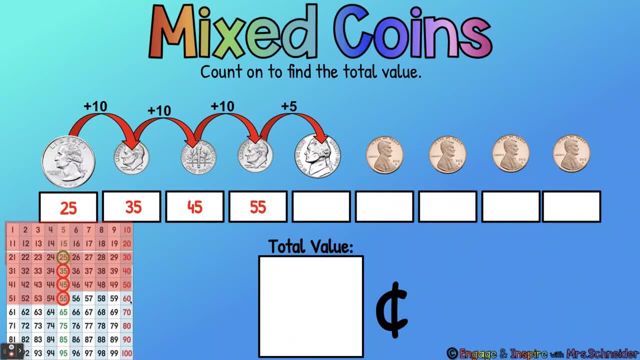 So 55 plus 5 is 60.. So 55 plus 5 is 60.. Sixty Sixty plus 1 is 61.. Sixty plus 1 is 61.. Sixty-two, Sixty-three, Sixty-four. 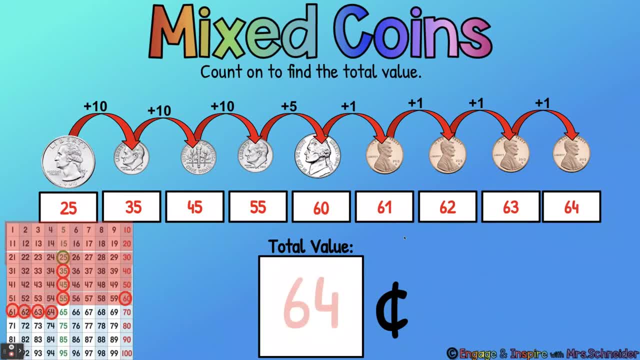 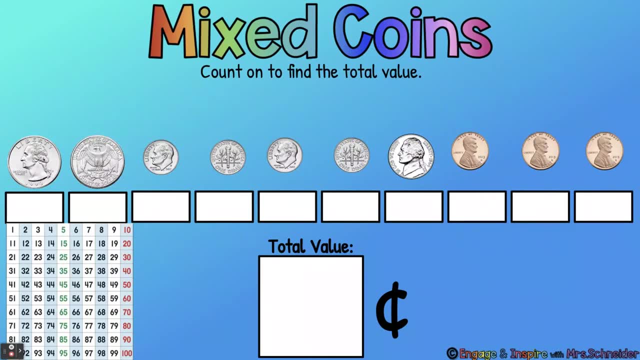 So our total value of these coins is 64.. So our total value of these coins is 64.. Sixty-four, Okay, here's another one. Are you guys having fun yet? One quarter is 25.. Two quarters is 50.. 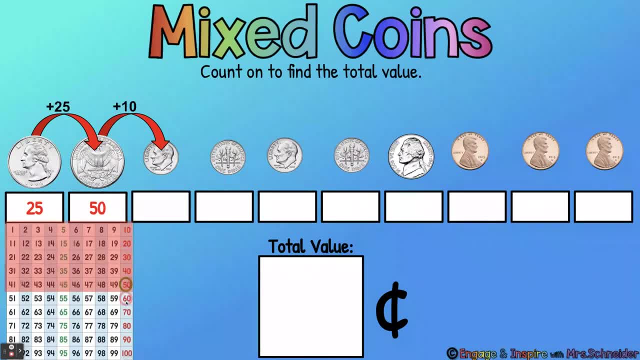 Okay, here's 50 on our chart. We're going to add 10.. 50 plus 10 is 60.. Plus 10 more is 70.. Plus 10 more is 80.. Plus 10 more is 90.. 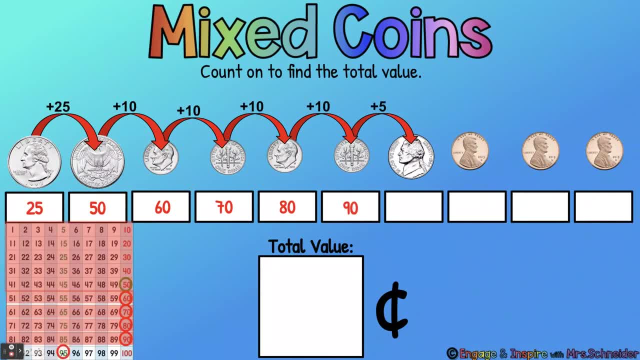 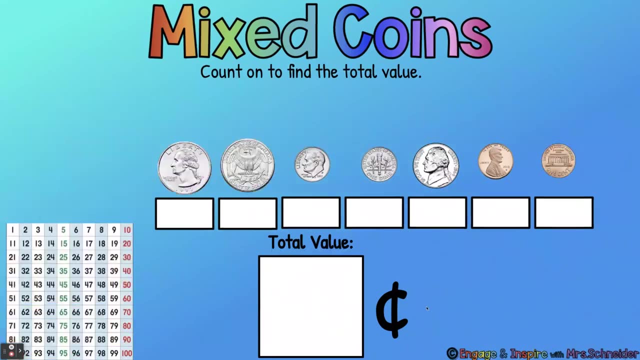 And 90 plus 5 is 95.. And 95 plus 1 is 96.. Plus 1 more is 97.. Plus 1 more is 98.. 98 cents is our total value. Here we go again. One quarter is 25.. 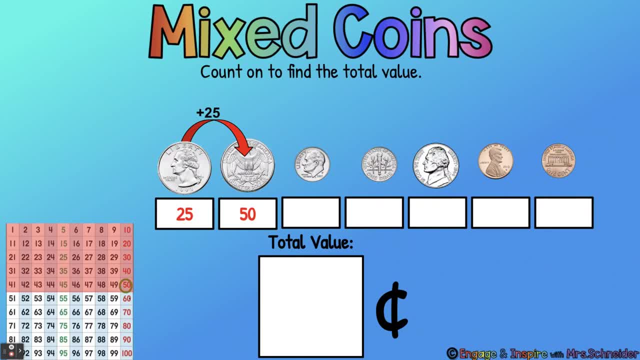 Two quarters is 50.. Okay, 50 plus 10 is 60.. Plus 10 more is 70.. And 70 plus 5 is 75.. Plus 1 more is 76.. Plus 1 more is 77.. 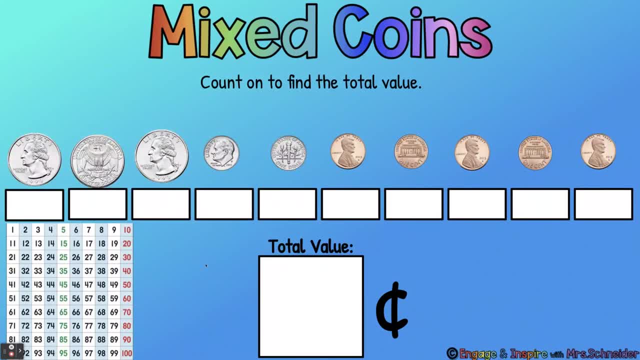 Awesome job, you guys. This one is 77 cents. Ooh, this one looks tough. Let's see, One quarter is 25.. Two quarters is 50.. Three quarters is 75. So let's look at 75 on our hundreds chart. 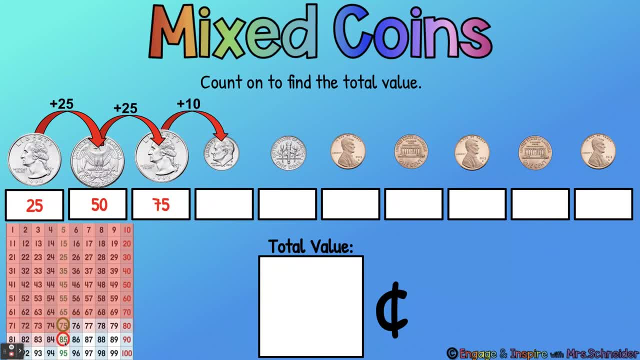 Okay, Add 10,. that'll put us at 85,, plus 10 more 95.. And now we're adding pennies Plus 1,, 96,, 97,, 98,, 99,, 100.. There's 100 cents there.